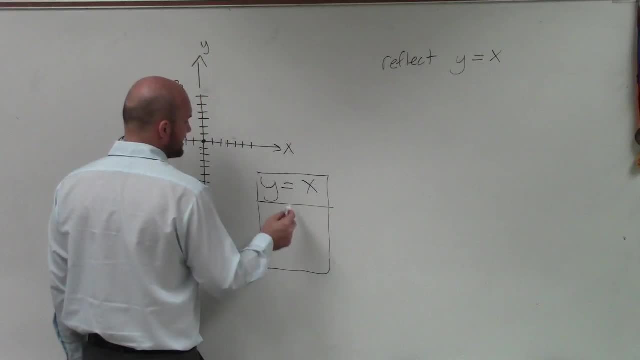 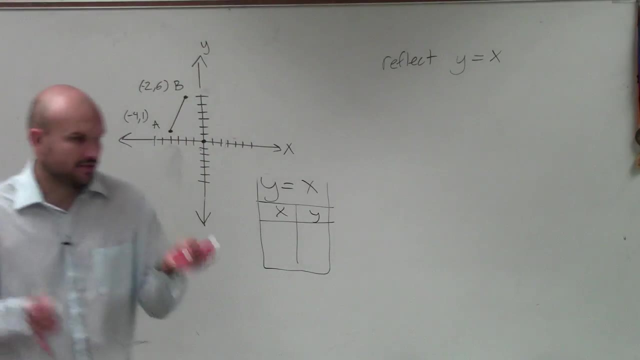 you guys learned how to graph lines, And when you're graphing lines, one thing you're told is: you can always create a table. You pick numbers for x, you plug them into the equation and then you find the values of y. So the equation that I want you to graph is: y equals. 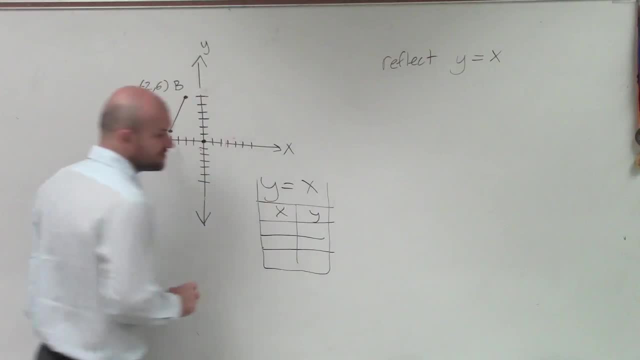 x. So a lot of times we just say, well, pick arbitrary values for x, So I'll do negative 3,, 0, and 3.. Well, whatever number I plug in for x, what is going to be the value for? 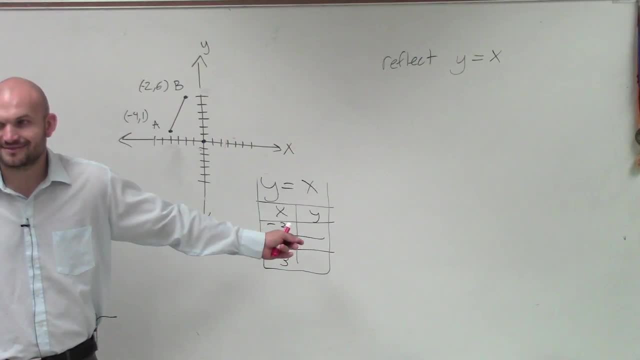 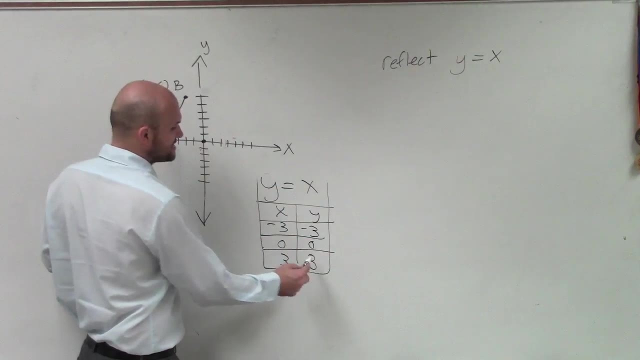 y The exact same, Because, remember, they have to equal each other, right? So therefore, that's negative 3,, that's 0, and that's 3.. So you might look and say: well, what is that graph going to look like That graph? 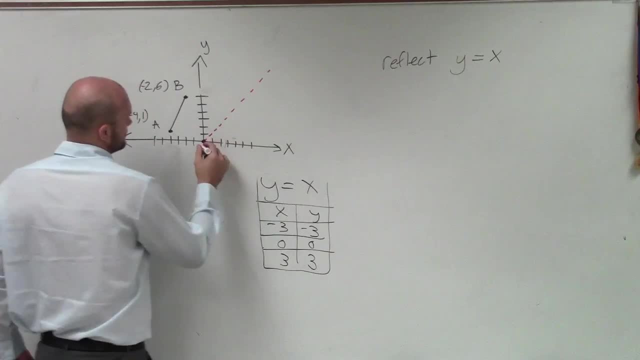 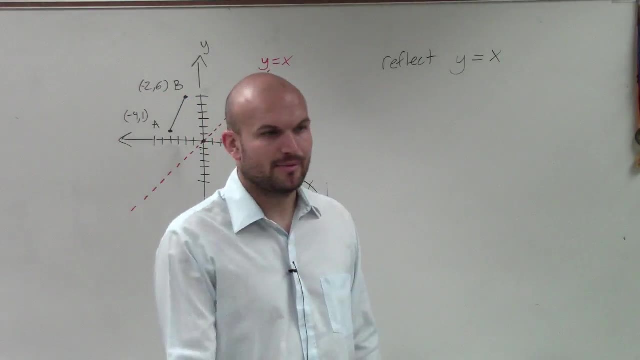 it's going to look like something like this, And I'm going to draw it as a dotted line, But that, ladies and gentlemen, is what we call the y equals x line. It's pretty much a nice straight, diagonal line that kind of cuts through your origin. So we need to 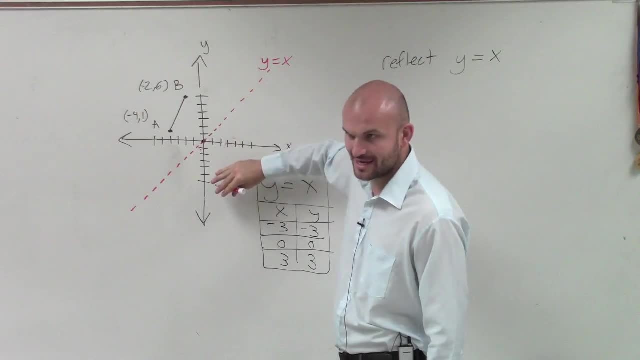 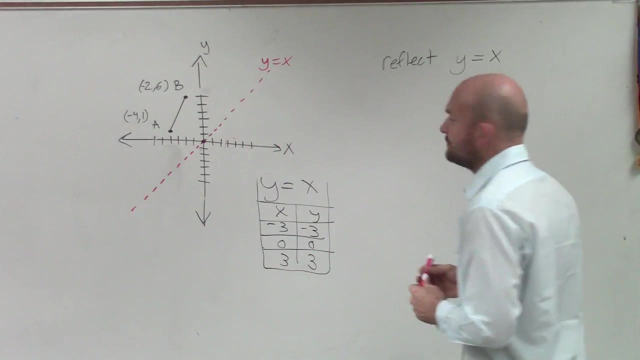 reflect this point over the y equals x line. So again, ladies and gentlemen, you can always think about it as like taking a sheet of paper and flipping it over to reflect it. Or, if you prefer to like the algebraic rule, you can take a sheet of paper and flip it over. 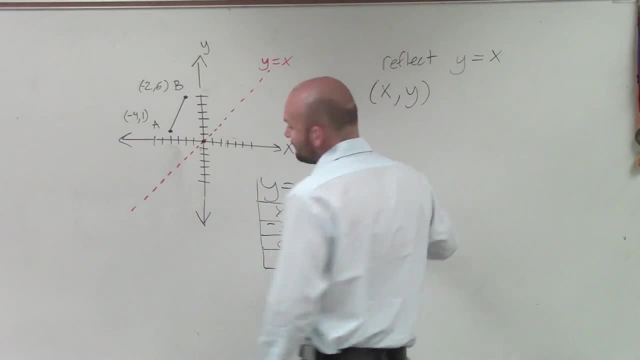 to reflect it. Here it is. So, on everything else we've previously done, we've talked about taking the opposite- right, Opposite of the sign or opposite of the sign- and keeping the other sign. good. Well, when we want to reflect the x equals y line or the y equals, 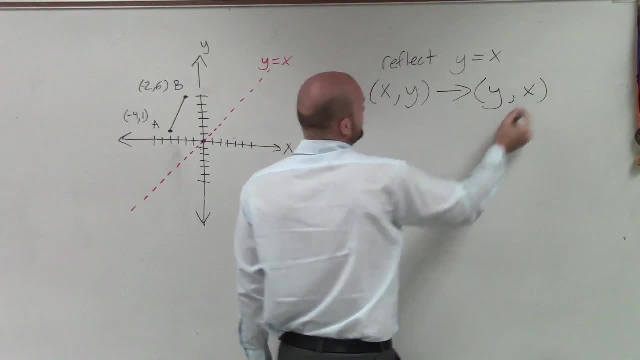 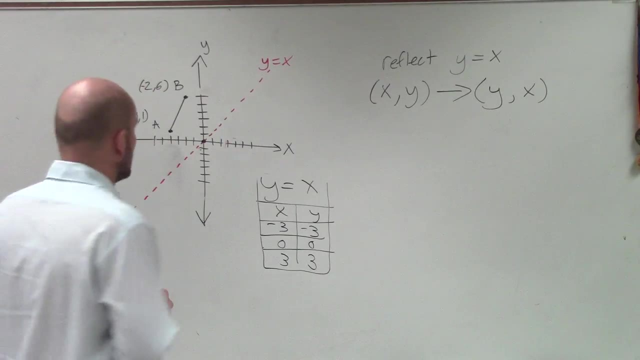 x line. we now just swap the variables. So this is a big distinction that you guys are going to want to make sure you are aware of. So let's look at our two points. So we have a which is negative 4.. 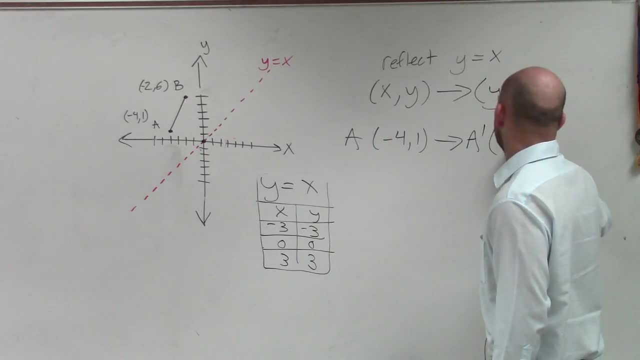 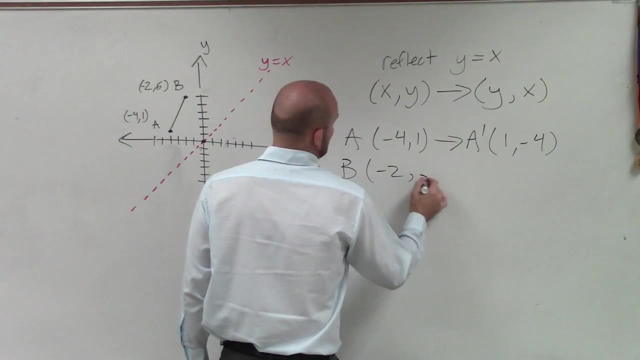 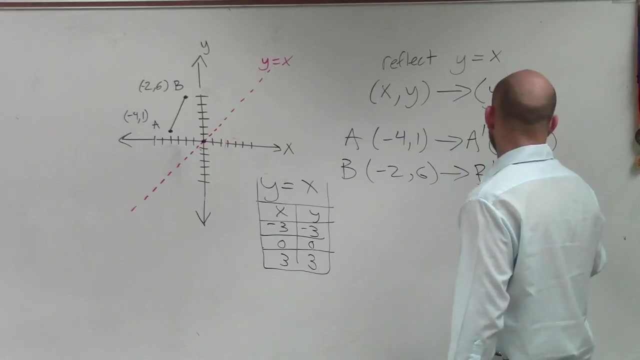 Well, now a prime is going to be 1 comma negative 4. You just swap them. And then here we have b, That equals negative 2 comma 6.. Again, ladies and gentlemen, all we're going to do now is just swap. So that's b prime equals 6 comma negative 2.. OK, So now we just